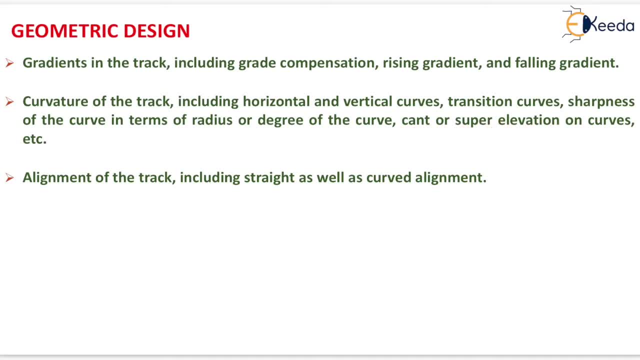 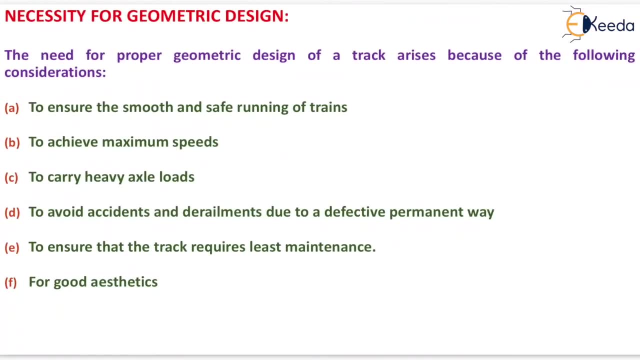 cant or super elevation on curves, etc. And the last one is alignment of the track, including straight as well as curved alignment- Now Necessity for Geometric Design. The need for proper geometric design of a track arises because of the following consideration. The first one is to ensure the smooth and safe running of trains. 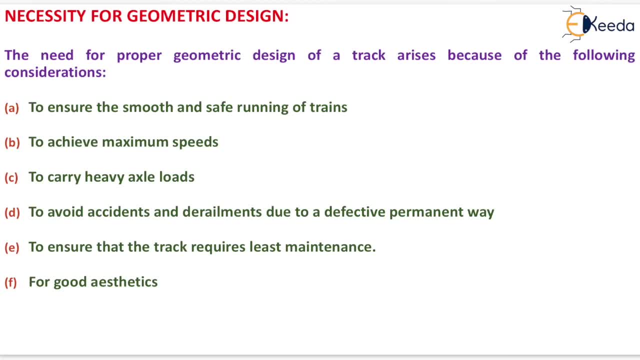 Next one is to achieve maximum speed. Another one is to carry heavy axle loads. The next one is to avoid accidents and derailments due to defective, permanent way. Another one is to ensure that the track requires least maintenance. And the last one is for good aesthetics. 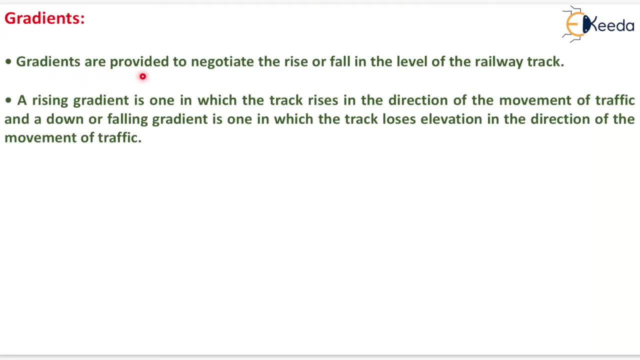 Now the next topic is the gradient Gradients are provided to negotiate the rise or fall in the level of the railway track. The next topic is the gradient Gradients are provided to negotiate the rise or fall in the level of the railway track. 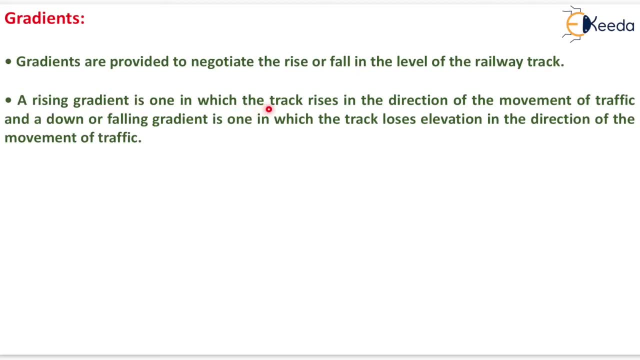 The next topic is the gradient. Gradients are provided to negotiate the rise or fall in the level of the railway track. A rising gradient is one in which the track rises in the direction of the movement of traffic, and a down or falling gradient is one. 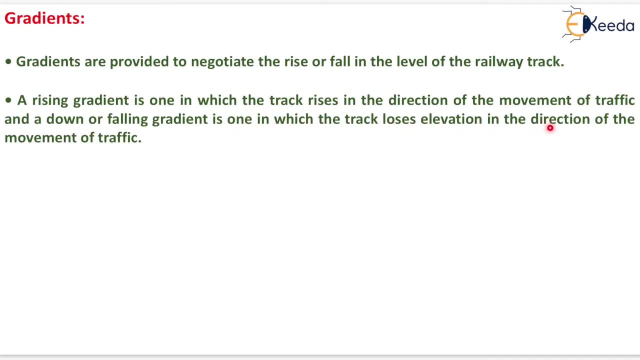 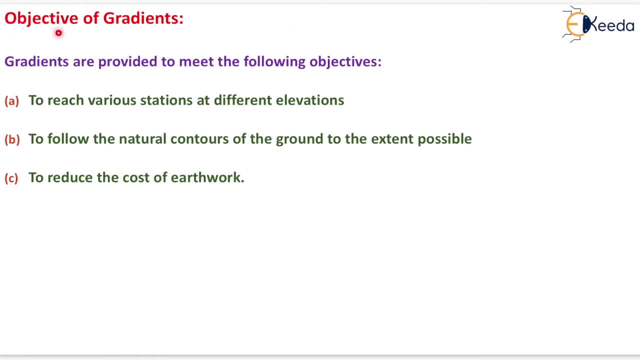 in which the track loses elevation in the direction of the movement of traffic. Now, objective of gradient. Gradients are provided to meet the following objective. The first one is to reach various stations at different elevations. Next one is to follow the natural contours of the ground. 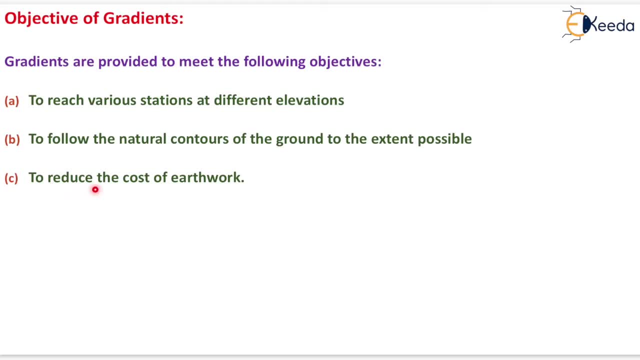 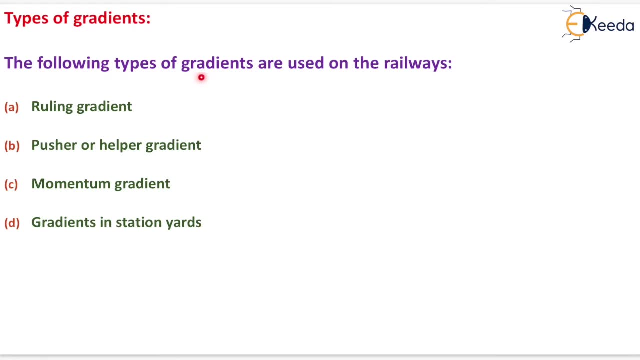 to the extent possible. and the last one is to reduce the cost of earthwork. Now the types of gradients. The following types of gradients are used on the railways: The first one is rolling gradient, Another one is pusher or helper gradient, The next one is momentum gradient and the last one is gradient in station yards. 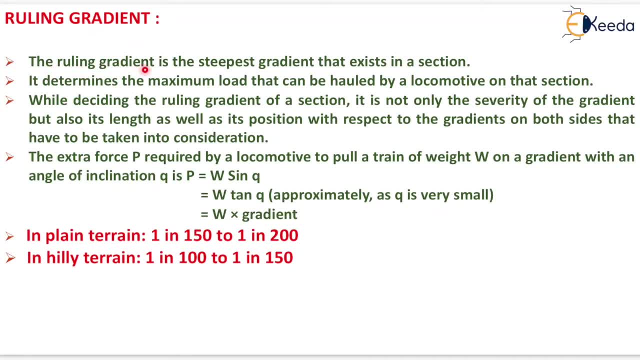 Now we will start with the rolling gradient. The rolling gradient is the steepest gradient that exists in a section. It determines the maximum load that can be hauled by a locomotive on that section. While deciding the rolling gradient of a section, 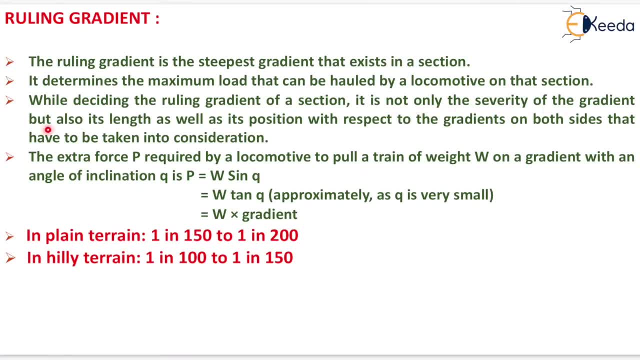 it is not only the severity of the gradient, but also its length, as well as its position with respect to the gradients on both sides that have to be taken into consideration. The extra force p required by a locomotive to pull a train is the ğı z. 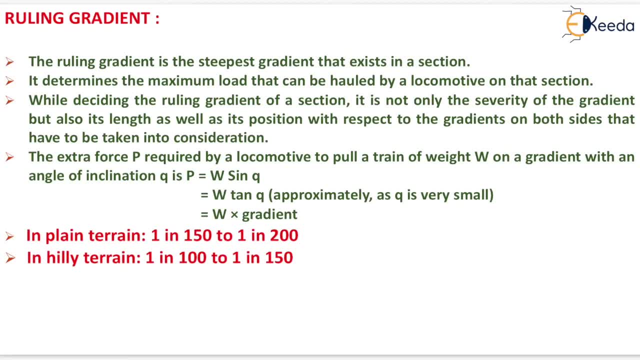 And in case of plane terrain, the. and in case of a hilly The轮Sanà fÄ XÑxÎx, neggÈkspÌ. eÅ r guex Мs Òu oÛn Õ æ ngÈr. A1 × u rég Waka — W lambda Büm ×7 ñ W deals with this degree. 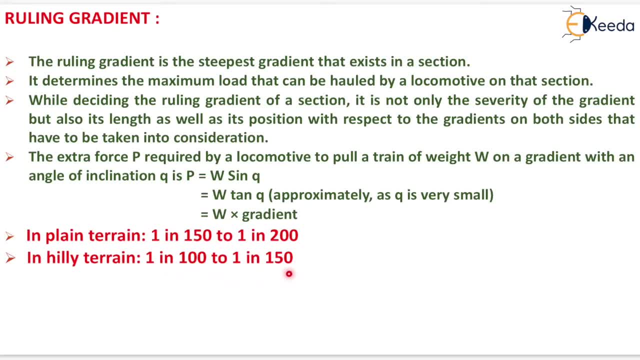 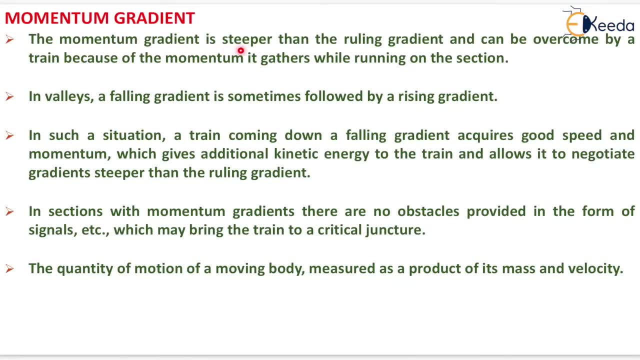 terrain. it will be equals to 1 in 100 to 1 in 150. now the next one is momentum gradient. the momentum gradient is steeper than the ruling gradient and can be overcome by a train because of the momentum it gathers while running on the 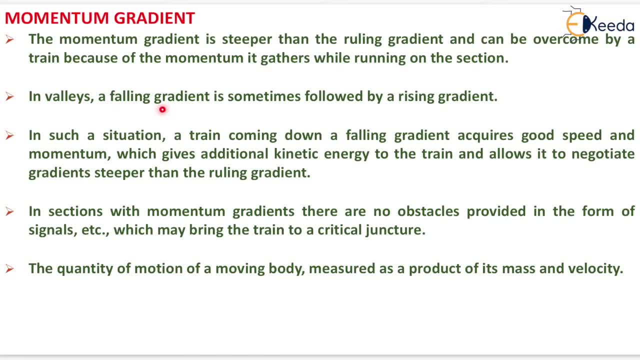 section. in valleys a falling gradient is sometimes followed by a rising gradient. in such a situation, a train coming down a falling gradient acquires good speed and momentum, which gives additional kinetic energy to the train and allow it to negotiate gradients- is cheaper than the ruling gradient in sections with. 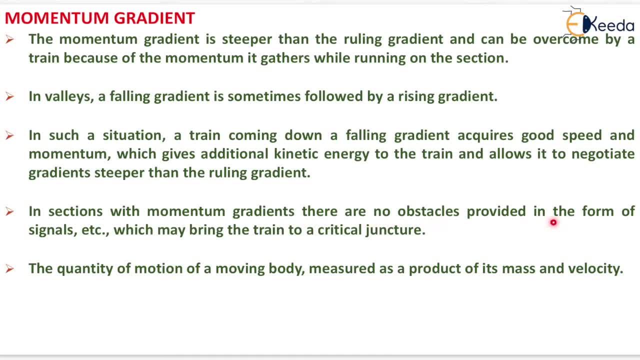 momentum gradients, there are no obstacles provided in the form of signals, etc. which may bring the train to a critical juncture. the critical juncture is the one which is the most effective in the case of the quantity of motion of a moving body measured as a product of its mass and 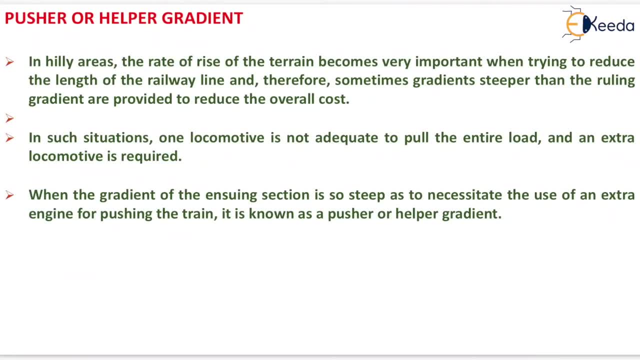 velocity. now the next is the pusher or helper gradient. in hilly areas, the rate of rise of the terrain becomes very important when trying to reduce the length of the railway line, and therefore sometimes gradients is cheaper than the ruling gradient are provided to reduce the overall cost. it means that when 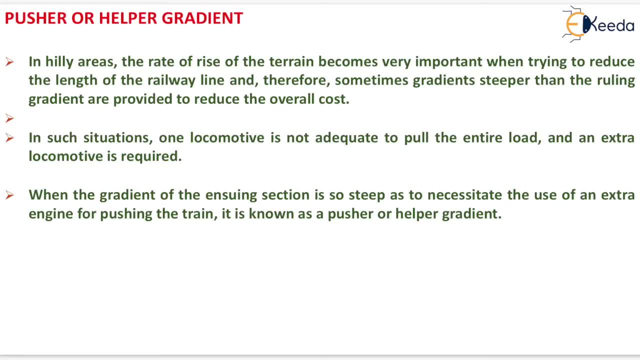 we want to reduce the cost of the construction, then we have to use the pusher or helper gradient in place of ruling gradient. in such situation, well, locomotive is not adequate to pull the entire load. an extra locomotive is required when the gradient of the section is so steep as to necessitate 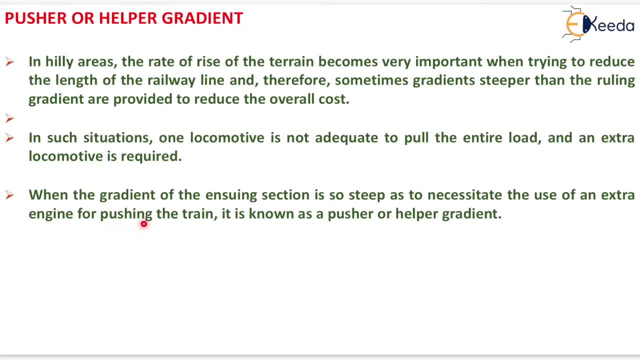 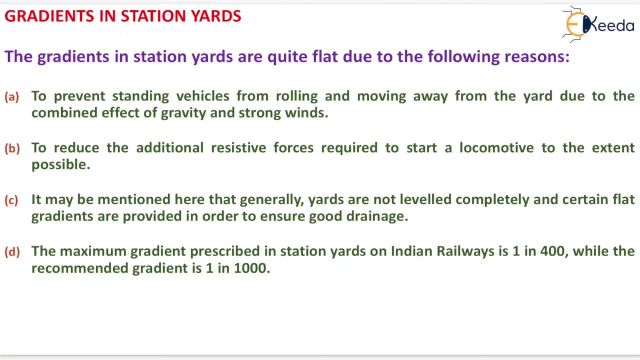 the use of an extra engine for pushing the train. it is known as pusher or helper gradient. now the next one is gradient in station yards. The gradients in station yards are quite flat due to the following reasons. The first one is to prevent standing vehicles from rolling and moving away from. 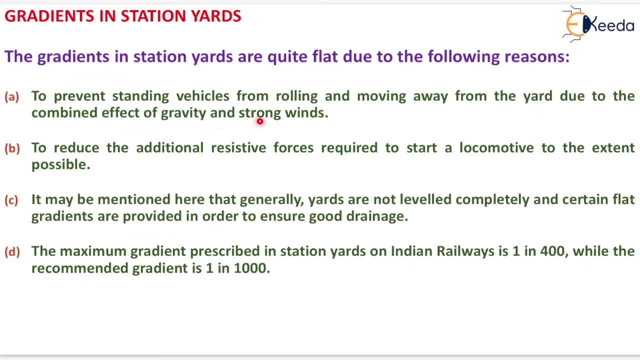 the yard due to the combined effect of gravity and strong winds, To reduce the additional resistive forces required to start a locomotive to the extent possible. It may be mentioned here that generally yards are not levelled completely and certain flat gradients are provided in order to ensure good drainage. The maximum gradient prescribed in station: 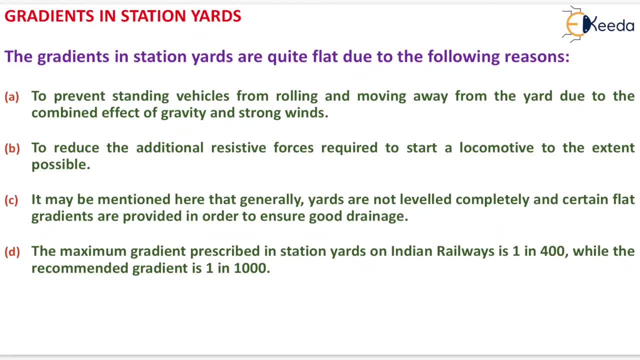 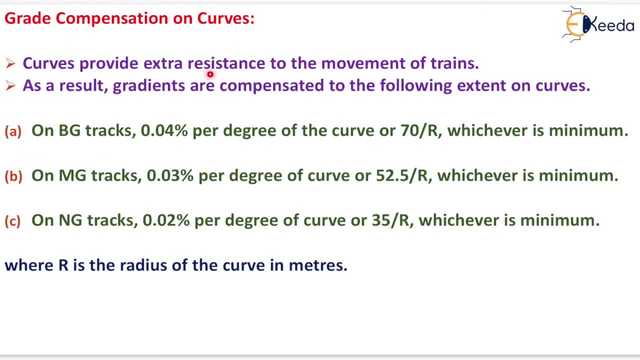 yards on Indian Railway is 1 in 400, while the recommended gradient is 1 in 1000.. Grade Compensation on Curves. Curves provided extra resistance to the movement of trains. As a result, gradients are compensated to the following extent on curves On broad. 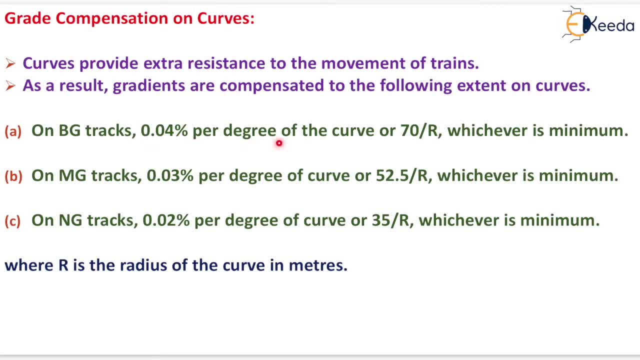 gauge tracks: 0.04% per degree of the curve or 70 by r, whichever is the maximum gradient is minimum. On meter gauge tracks: 0.03% per degree of curve or 52.5 upon r, whichever is minimum. On narrow gauge tracks: 0.02% per degree of curve or 35 upon r, whichever. 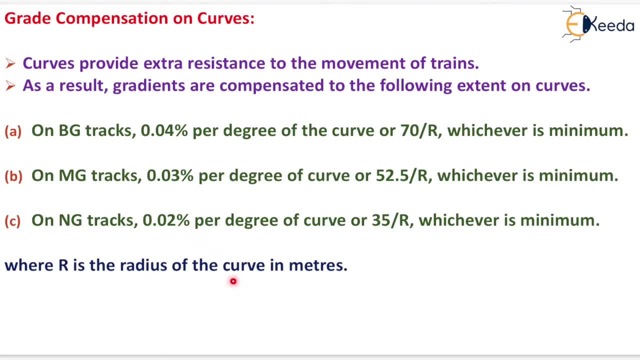 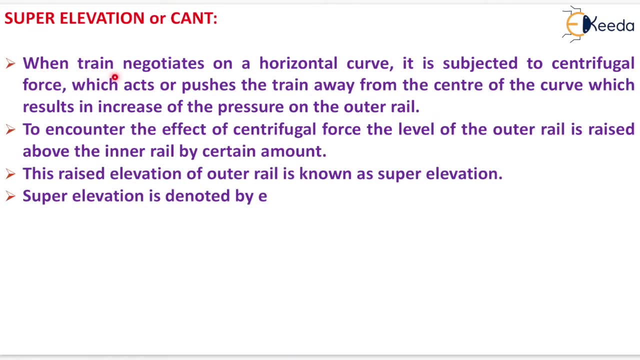 is minimum, Where r is the radius of the curve in meter. Now next one is the Super Elevation, or Kent. When train negotiates on a horizontal curve, it is subjected to centrifugal force, which acts or pushes the train away from the centre. 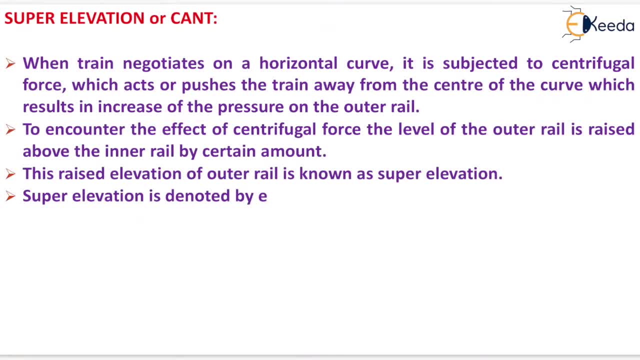 of the curve, which results in increase of the pressure on the outer wheel. Now, to counter the effect of centrifugal force, the level of the outer rail is raised above the inner rail by certain amount. This raised elevation of outer rail is known as super elevation. 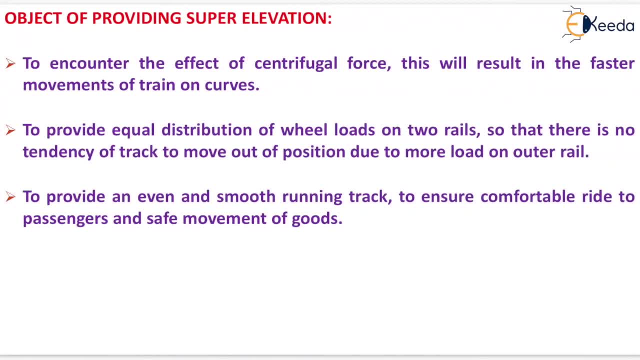 Super elevation is denoted by E Objects of providing super elevation To encounter the effect of centrifugal force. this will result in the faster movement of train on curves. To provide equal distribution of wheel loads on two rails so that there is no tendency of track to move out of position. 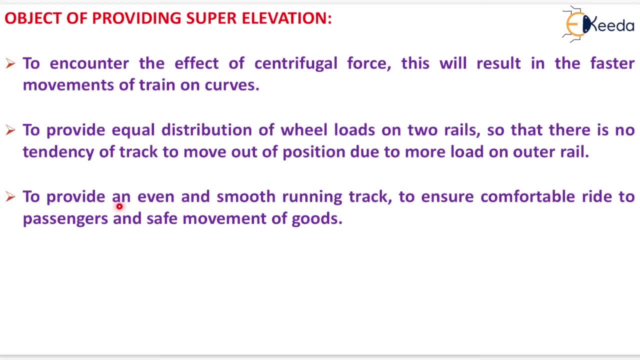 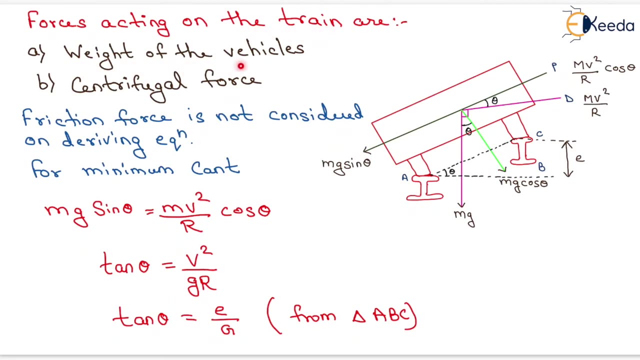 due to more load on outer rail, To provide an even and smooth running track and to ensure comfortable ride to the passengers and safe movement of goods. Now, forces acting on the train are: first one is weight of the vehicle and the next one is centrifugal force. Here the train is shown like this: and this is the rail and this: 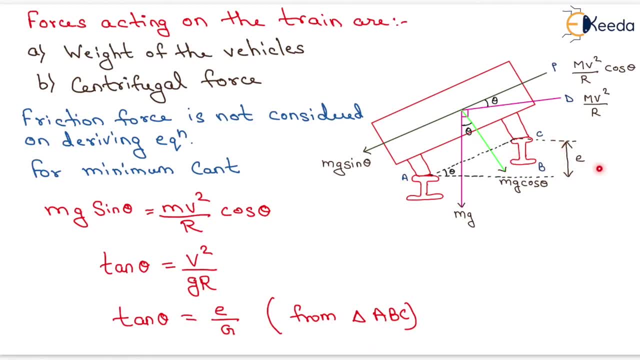 is the difference in the level of two rails, which is known as super elevation. It is denoted by E. Now this is the centrifugal force: mv square by r, and this is the weight of the vehicle. that is mg. Now, this angle is theta, so this angle is also theta, and this angle is also theta Now. 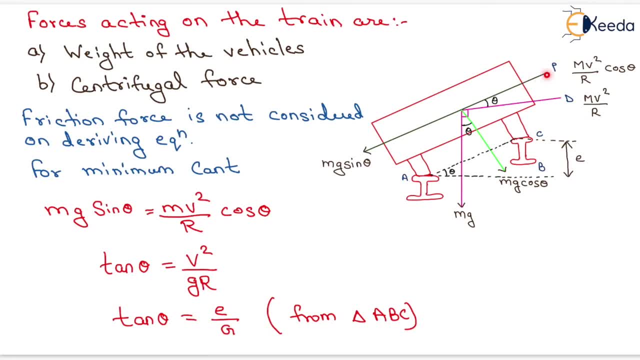 the component of this mv square by r on this axis will be equal to mv square by r into cost theta. Now the component of mg on this axis will be equal to mg cost theta and on this axis will be equal to mg sine theta. Now friction force is not considered. on deriving equation. 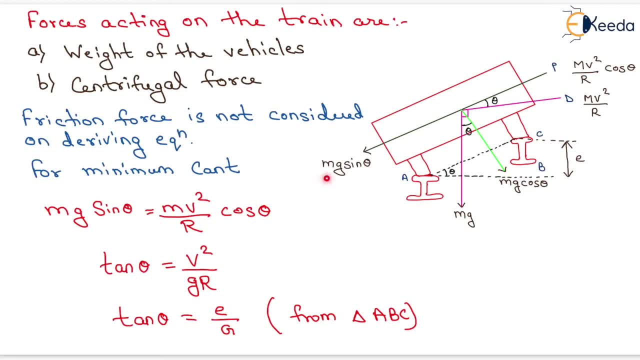 for minimum Can mg sine theta, that is, this will be equals to mv square by r. cos theta, which is shown here Now, sine theta upon cos theta, will be equals to tan theta and it will be equals to v square upon gr and m and m- cancel out Now from triangle ABC. tan theta will be equals to e by g. that is the. 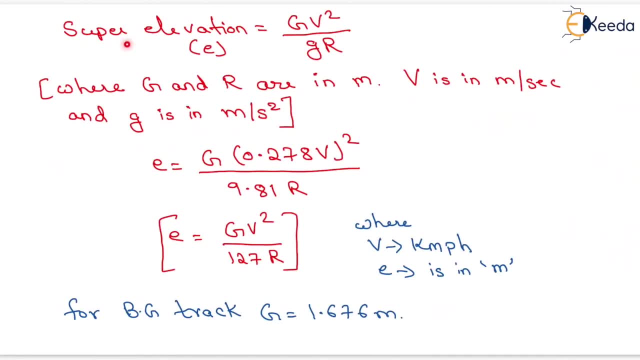 distance g Now super elevation, e will be equals to gv square upon small g into r, where capital g and r are in meter and v is in meter per second and small g is in meter per second square. Now e will be equals to. we have to convert the value of capital v in terms of meter per second. 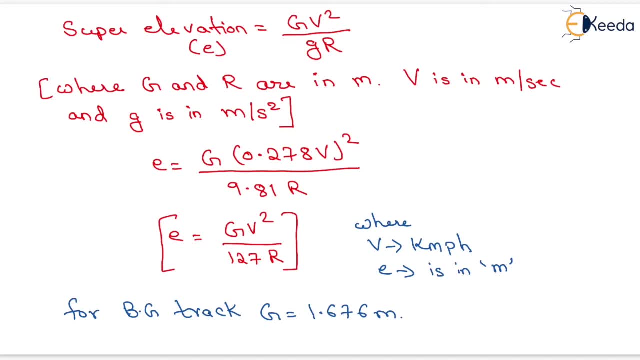 from kilometer per hour. So we need to multiply here the value of v by 0.278.. So the formula will be equals to g into 0.278. v whole square upon 9.81. r, The value of small g will be equals to 9.81.. After solving this we will have the value of super elevation, or. 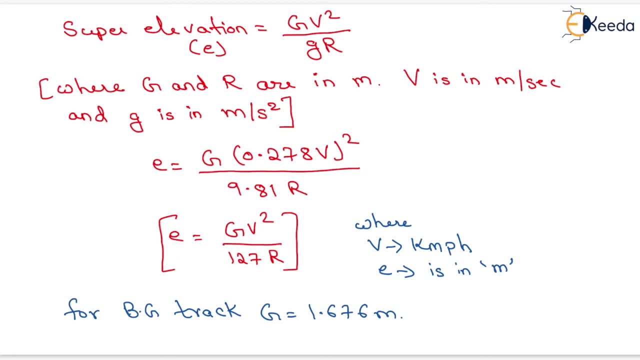 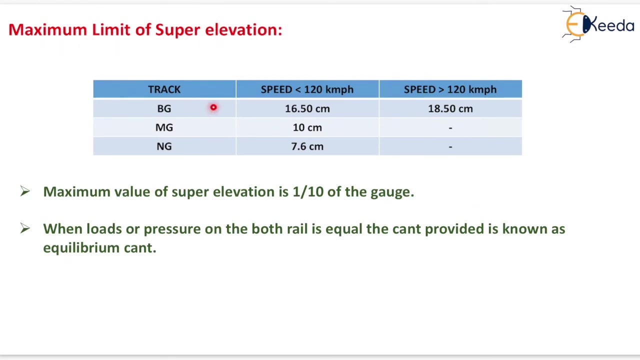 cant, that is small. e will be equals to gv, square upon 127 r, where v is in kilometer per hour and e is in meter. Now for broad gauge track, g will be equals to 1.676 meter, Now maximum limit of super elevation for broad gauge track. if 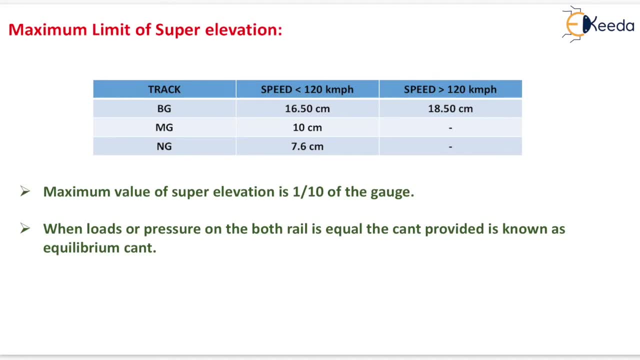 speed is less than 120 kilometer per hour, then maximum super elevation will be equals to 16.50 centimeter, and if speed is greater than 120 kilometer per hour, then maximum super elevation will be equals to 18.50 centimeter. Similarly for meter gauge and for: 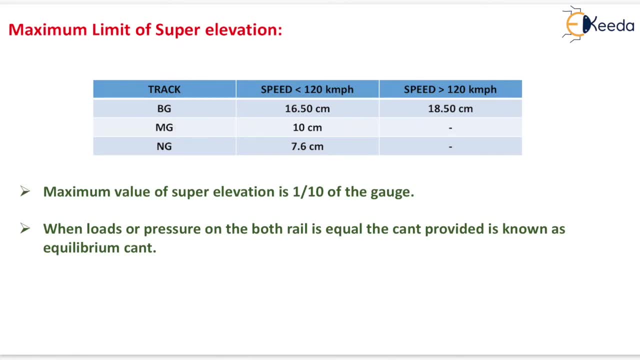 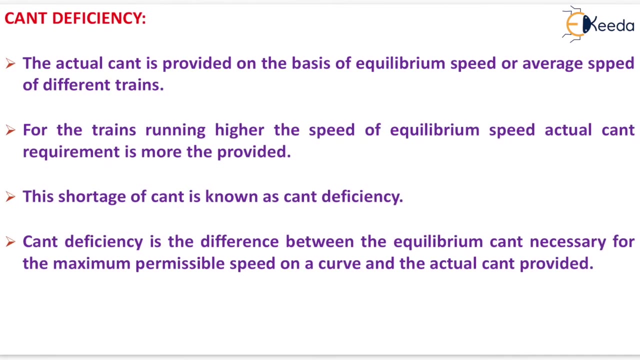 narrow gauge. it is shown here Now. maximum value of super elevation is 1 by 10 of the gauge. When loads or pressure on the both rail is equal, the cant provided is known as equilibrium cant. Now the next one is cant deficiency. The actual cant is provided on the basis of equilibrium. 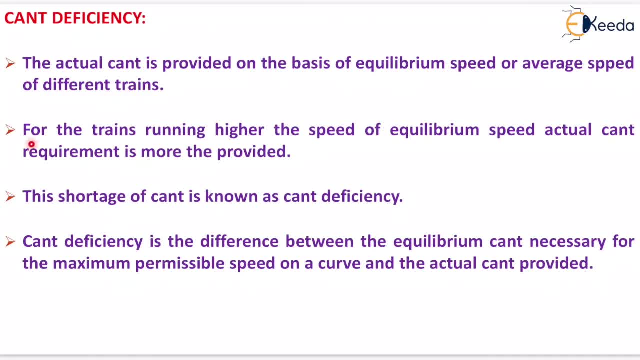 speed or average speed of different trains. For the trains running higher the speed of equilibrium speed, actual cant requirement is more than provided. This shortage of Cant is known as cant deficiency. Cant deficiency is the difference between the equilibrium cant necessary for the maximum permissible speed on a curve and the actual cant provided. 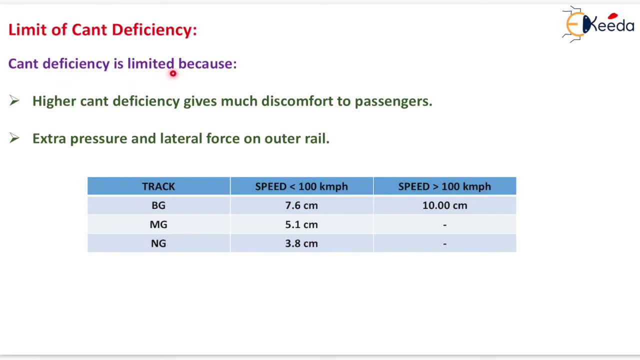 Now limit of cant deficiency. Cant deficiency is limited because higher cant deficiency gives much discomfort to passengers and extra pressure and lateral force on outer rail. Now in first column of this table track is shown. In second column speed less than 100 km per hour. 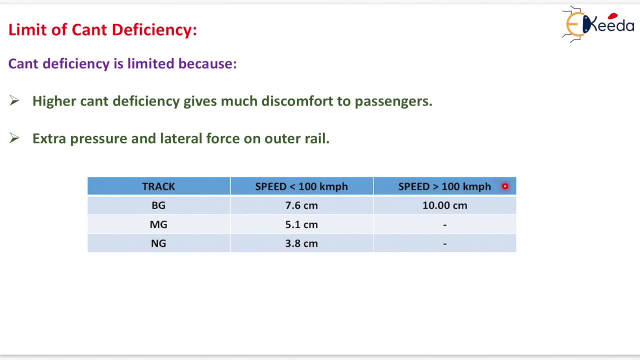 and in third column, speed greater than 100 km per hour is shown. Now for broad gauge, cant is limited to 7.6 cm when the speed is less than 100 km per hour and 10 cm when speed is greater than 100 km per hour.